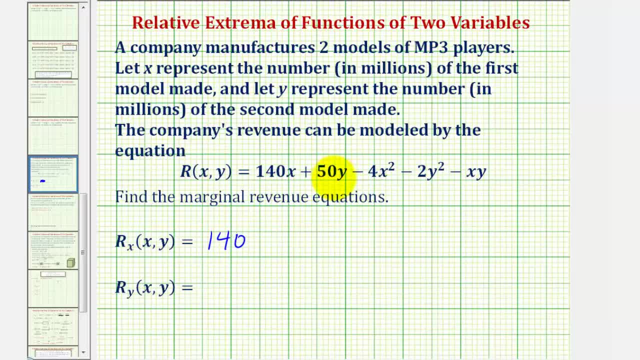 plus the derivative of 50y with respect to x would be zero, since we're treating y as a constant, minus the derivative of four x squared with respect to x. that would be minus eight x and then minus the derivative of two y squared. 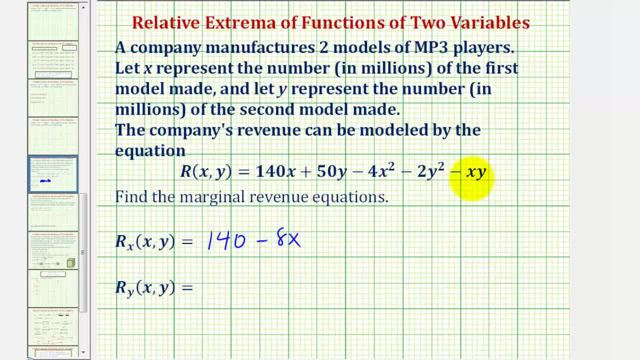 with respect to x would be zero, and then minus the derivative of xy. with respect to x, that would be minus y. And now for the partial derivative. with respect to y, we'll differentiate with respect to y, treating x as a constant. 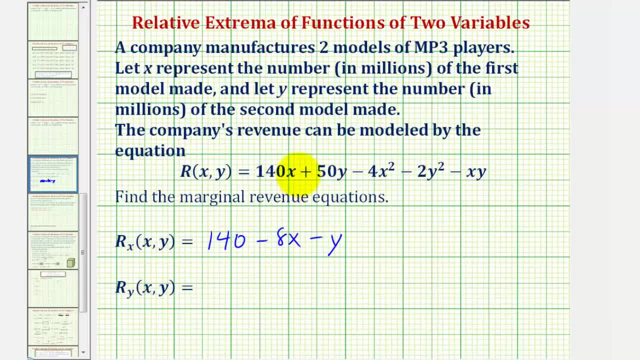 And therefore the derivative of 140x with respect to y would be 0,, plus the derivative of 50y with respect to y, that'd be 50, minus. the derivative of 4x squared with respect to y would be 0,, minus the derivative of 2y squared with respect to y. 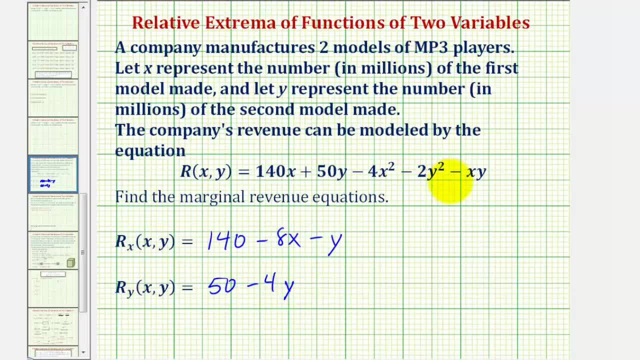 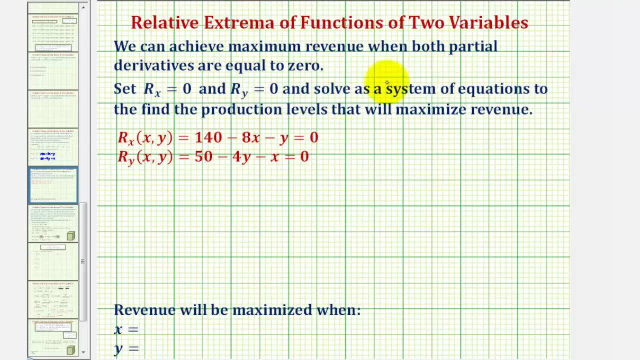 that would be minus 4y, and then minus the derivative of xy with respect to y would be minus x. So here's the first part of our question. For the second part, we can achieve maximum revenue when both partial derivatives are equal to 0.. 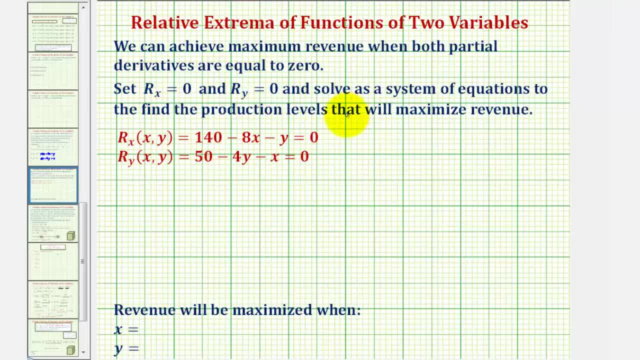 So we want to set our partial derivatives equal to 0 and solve as a system of equations to find the production levels that will maximize revenue. So here are the partial derivatives from the first slide. Notice how I set them equal to 0, and now we'll solve this as a system. 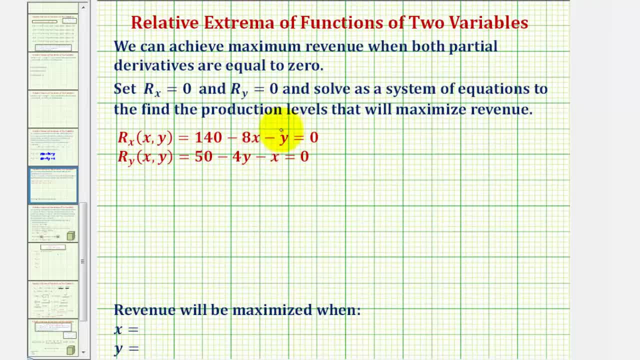 So to solve this system, let's use substitution. Let's go ahead and solve this first equation here for y. Notice, if we add y to both sides of the equation, we could write this as y equals 140 minus 8x. So now we'll substitute 140 minus 8x for y in the second equation and then solve for x. 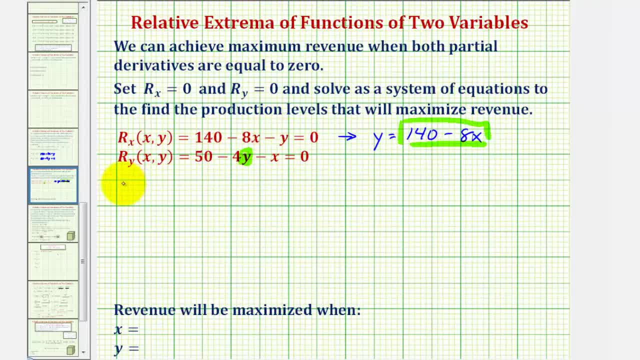 So, making the substitution, we would have 50 minus 4 times the quantity 140 minus 8x, and then minus x equals 0.. Let's clear the parentheses and solve for x. So we'd have 50, this would be minus 560 plus 32x. 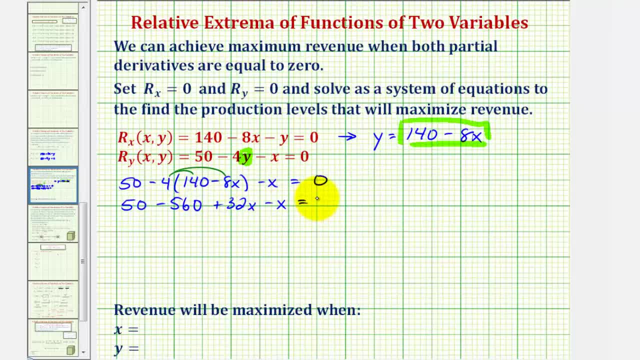 minus x equals 0. So we'd have 4 times the quantity 140 minus 8x, and then minus x equals 0. So combining like terms, we have negative 510 plus 31x equals 0.. Add 510 to both sides. 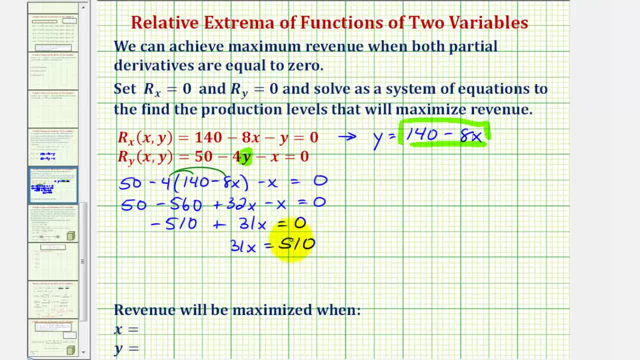 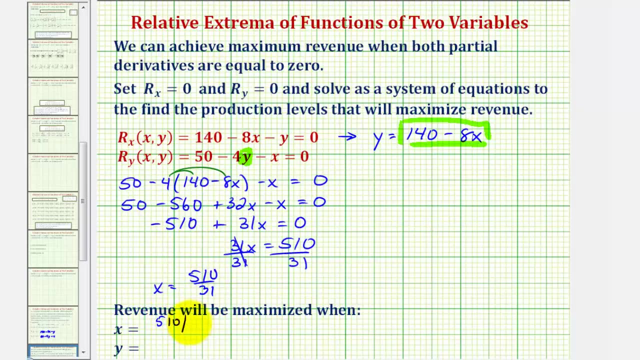 That would give us 31x equals 510, divide by 31.. So the exact value of x that would maximize revenue is 510 divided by 31.. Let's go ahead and write that here. Let's also look at our decimal approximation. 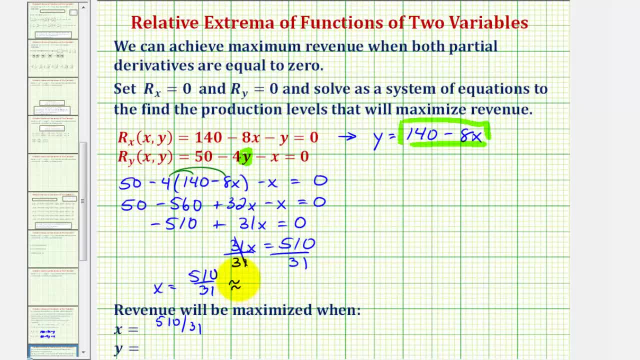 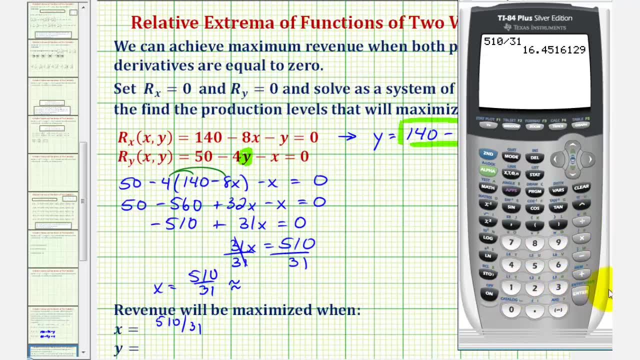 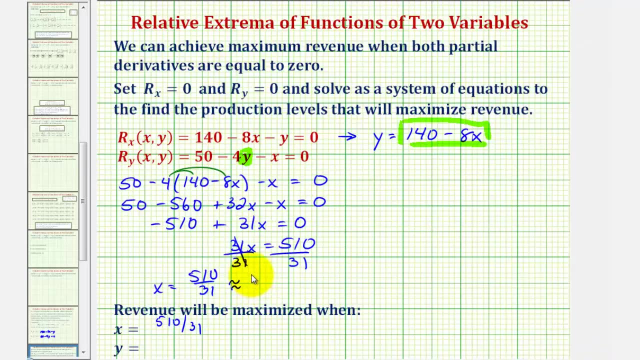 because, remember, this represents the production level in millions of MP3 players. So 510 divided by 31,. if we run to four decimal places, this would be approximately 16.4516.. Notice: in this form we can tell that the production level is approximately 16.4516 million iPods for Model 1.. 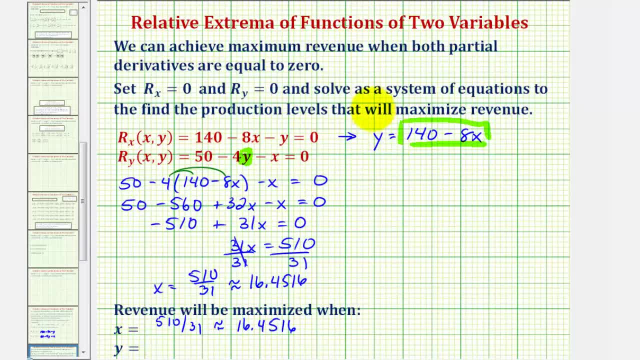 And then to find the production level for the second model, we'll determine y, where y is going to be equal to 140 minus 8 times the exact value of 510 divided by 31.. So we'll get the exact value and then we'll get our decimal approximation. 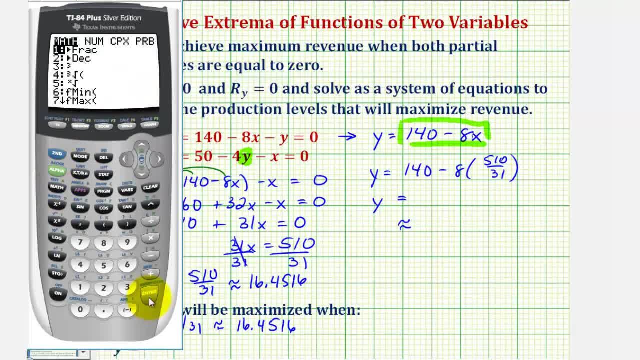 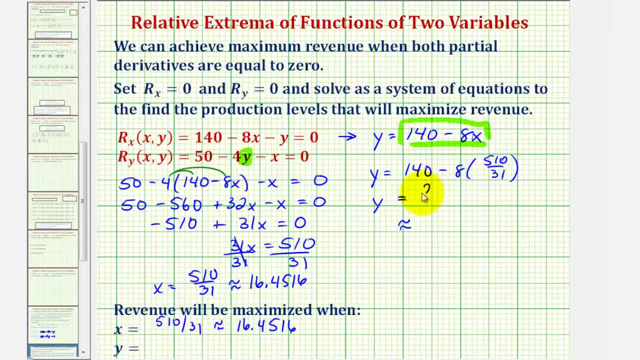 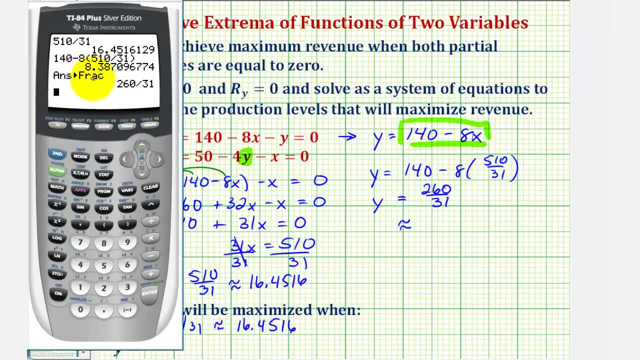 So here's the decimal approximation. If we press math, enter, enter, we can get the exact value of 260 divided by 31.. So we'll get the exact value of 510 divided by 31.. Well, the decimal approximation to four decimal places would be approximately 8.3871. 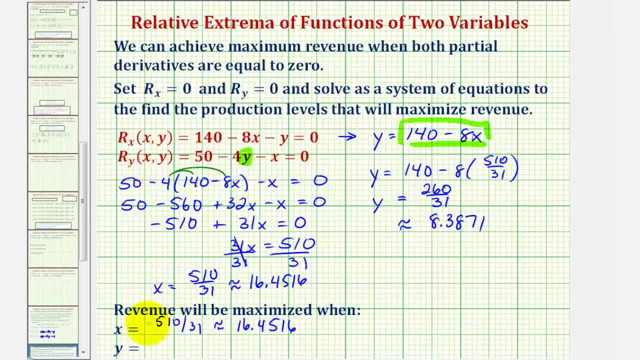 So we'll get. the exact value would be 260 divided by 31,, which is what we should enter, But to better understand this, it's approximately 8.3871.. And again, these are the production levels in millions of iPods. I hope you found this helpful.